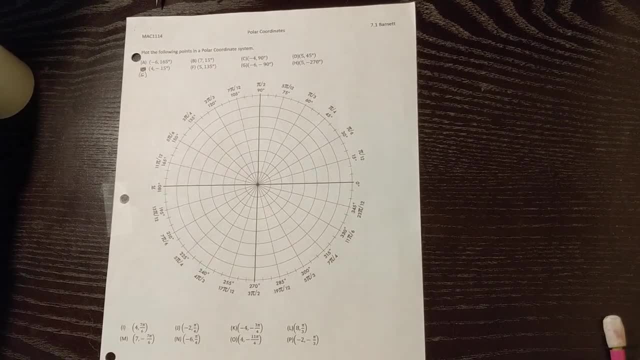 This video is about how to graph points in the polar coordinate system. So on your handout you have a polar coordinates that are graphed, that's given and it looks a lot like the unit circle, but there are more degree, there are more places marked on this than your unit circle. so first I want you 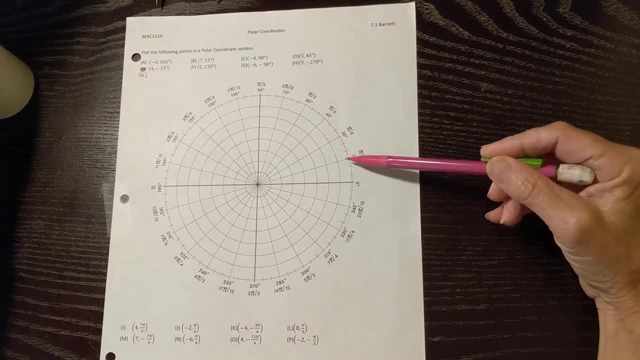 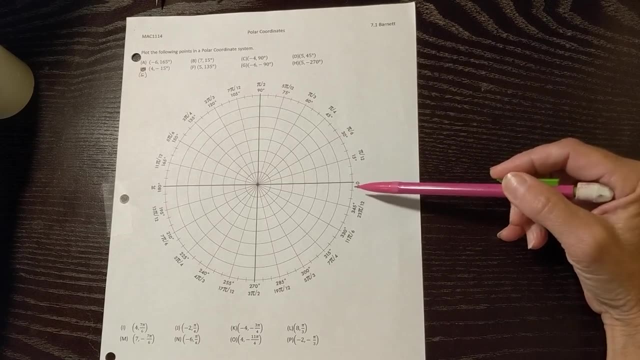 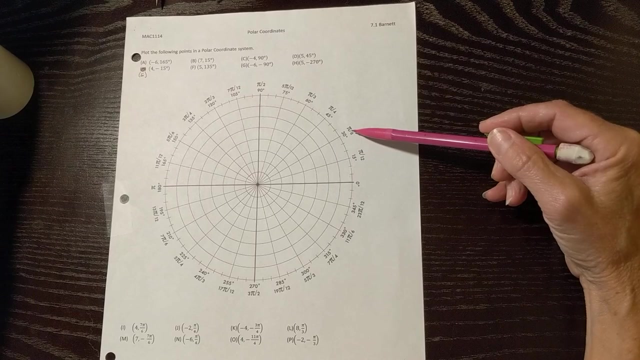 to look at this and just be aware that we're normally the first place that is marked as pi over 6. they have it split up into, excuse me, 15 degree increments, so the first place they have marked is 15 degrees, not 30 degrees, which is pi over 12. so just be aware of that. this is pi over. 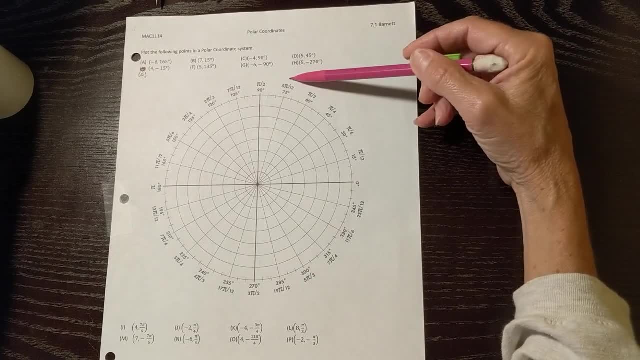 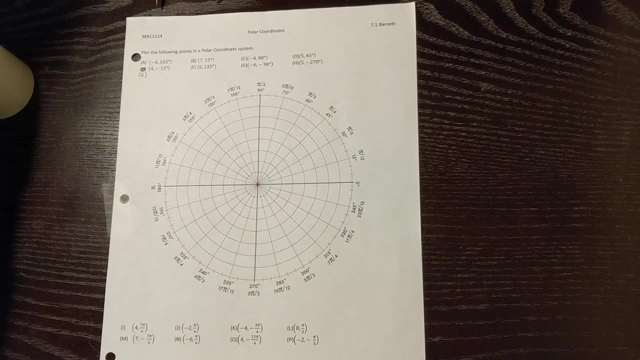 6 pi over 4 pi over 3, 5 pi over 12. they have these little every 15 degrees, so it's a little bit different. that just means you have to be kind of careful. we're gonna graph these points I have marked on the worksheet A through E. 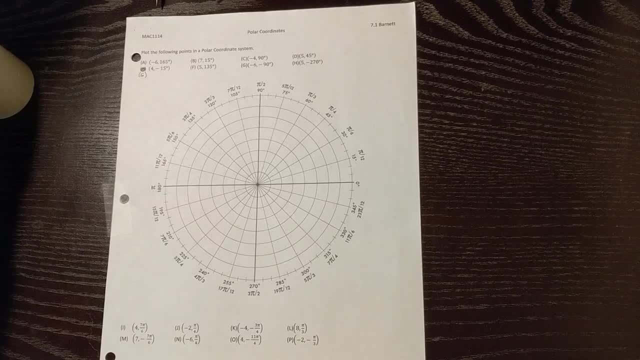 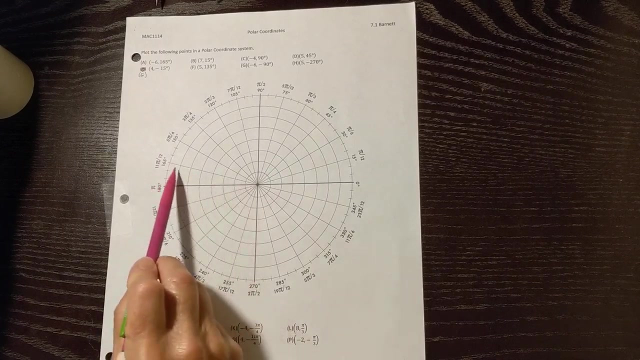 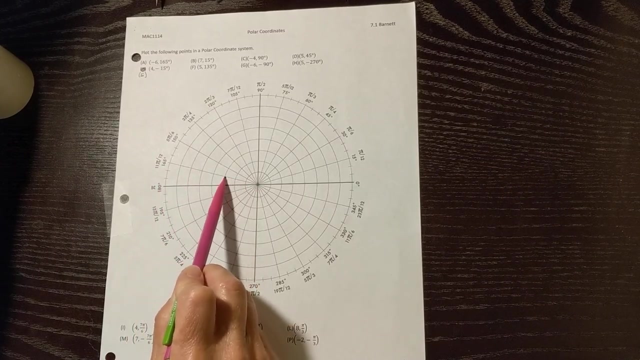 and so let's begin with A, which is negative six 165 degrees. So what you should do to graph the point negative six 165 degrees is find 165 degrees. So right, here is 165 degrees. Now, if if we had a positive number, we would move towards in the direction of 165 degrees, but we have a negative. 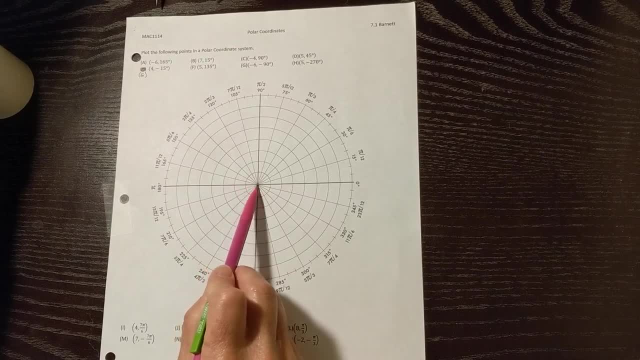 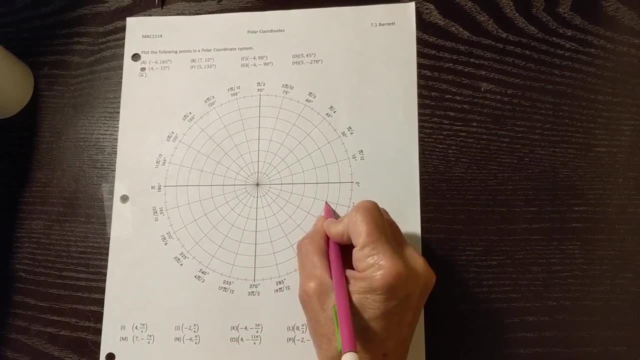 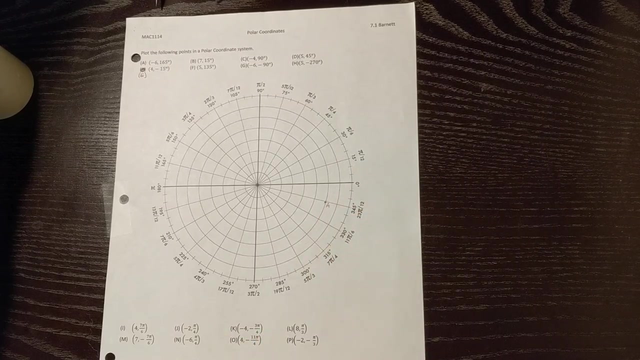 six. so that means we're gonna go 185 degrees, degrees across from that, and we're going to go six. that way, one, two, three, four, five, six, and this will be the first place. we put something- and this is point a and B is 7, 15 degrees. so go to 15 degrees, and so here is 15 degrees, and 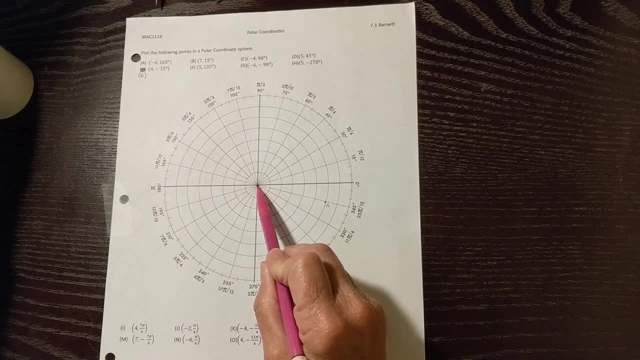 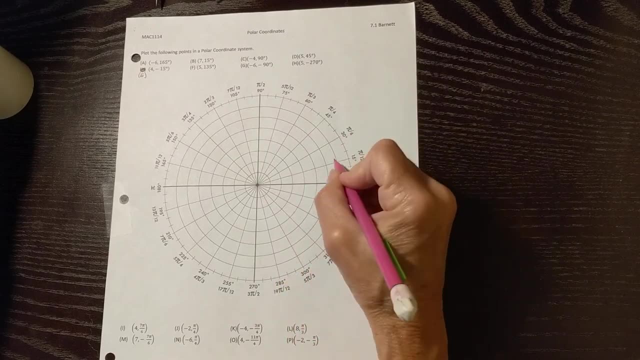 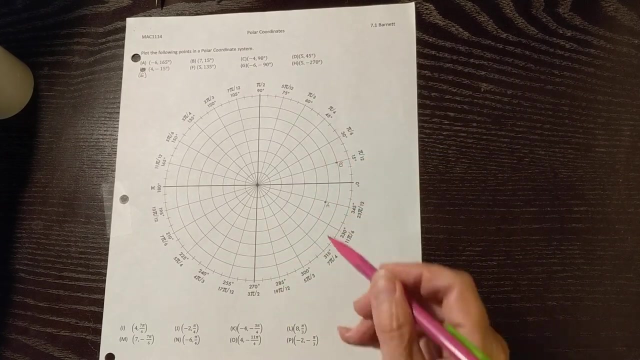 then we're going to move up the grid. seven marks in the direction of 15 degrees, because seven is positive. one, two, three, four, five, six, seven, just like that. this is B. C is negative. 490 degrees go to 90 degrees, which is right here. but 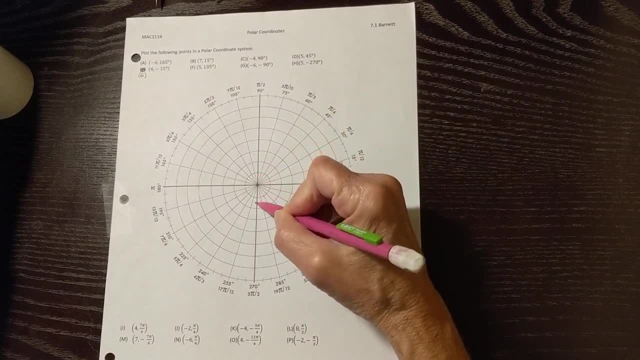 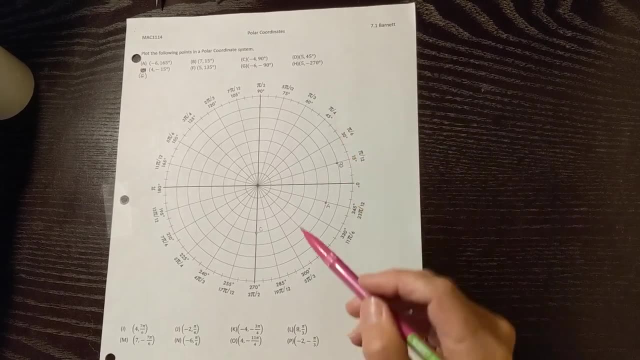 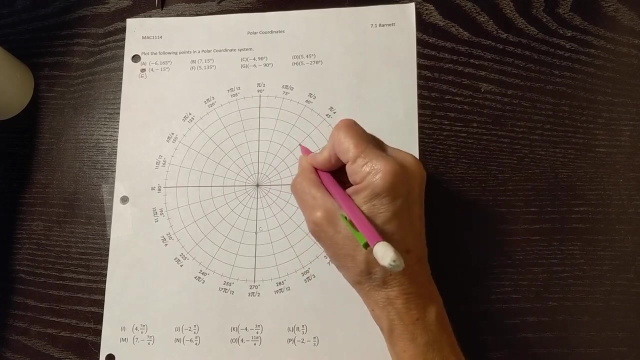 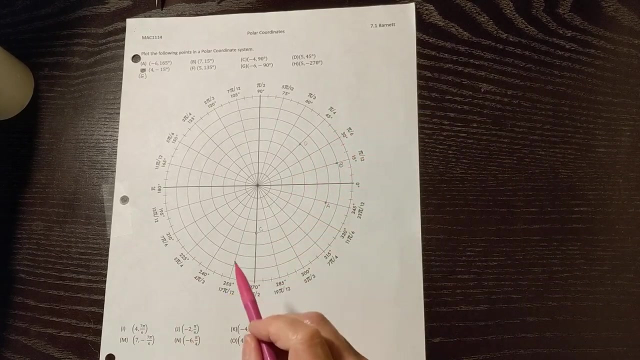 since it says negative 4, we're going to go on the opposite direction. one, two, three, four- this is where C will be. D is five, 45 degrees. find 45 degrees right here. we're going to go up one and now it will be B: two, three, four, five, and this will be D. e is for negative 15. go to negative 15. okay, this is where. 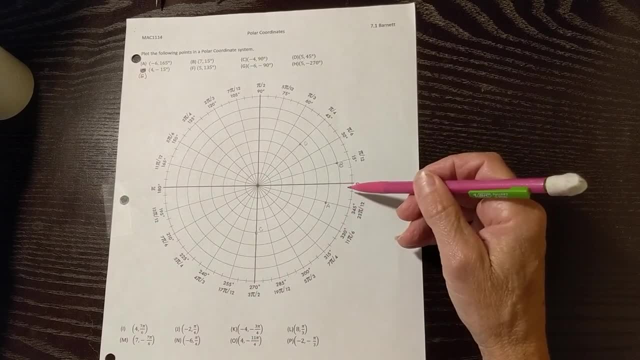 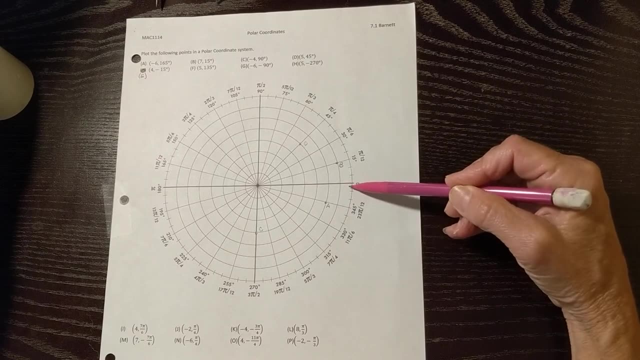 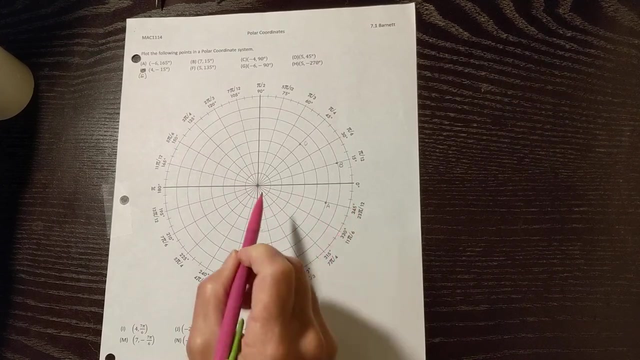 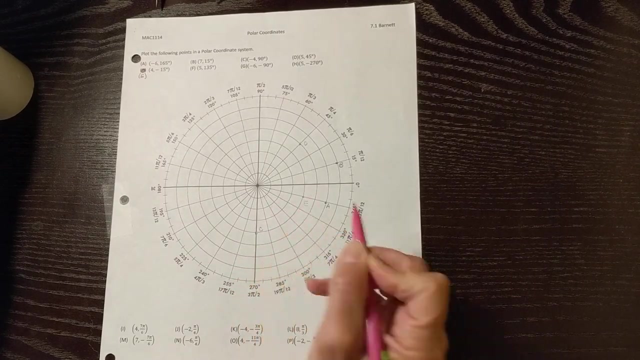 people get. I don't know, something goes funny with them, but negative 15 degrees is if you're moving clockwise 15 degrees. so this, right here, this is negative 15 degrees. so go to negative 15 degrees. and they want us to go four units out: one, two, three, four. this is where E is okay. five, 135 find. 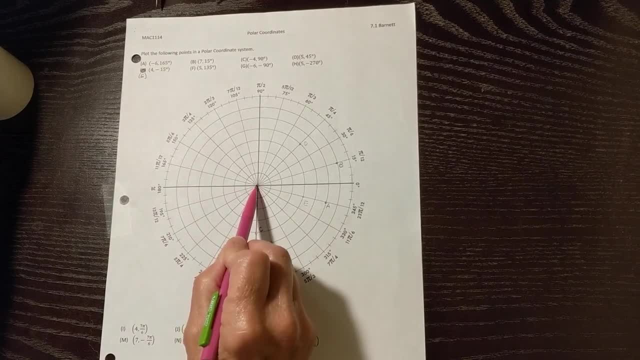 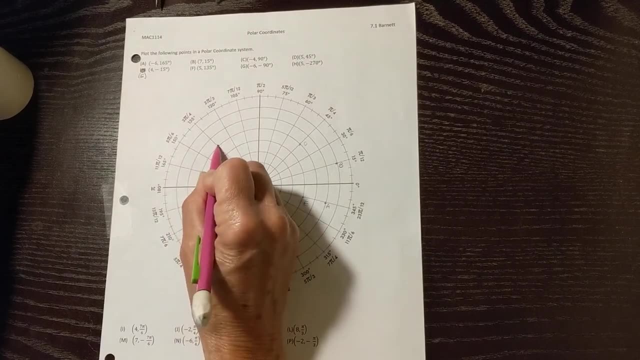 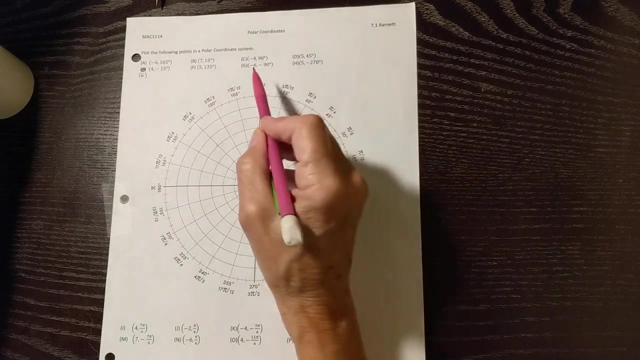 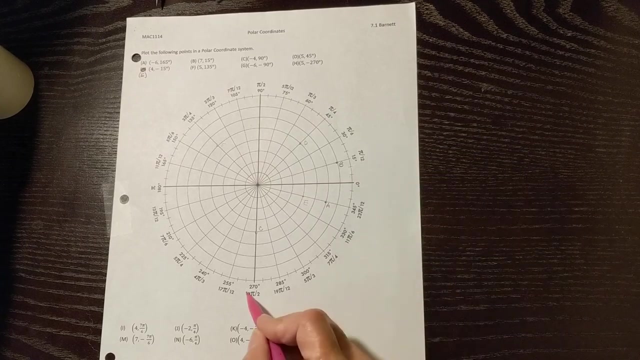 135 right here, and we're going to go up one, two, three, four, five, and so this is going to be F right here. okay, G is negative six negative ninety. so first go to the angle negative negative 90.. Where is negative 90?? Well, go clockwise: 90 degrees. So this 270 is 90 degrees. 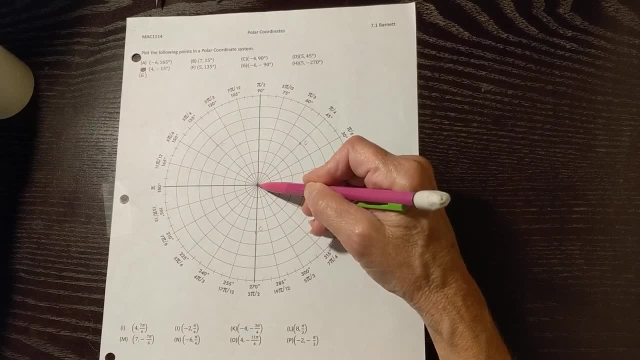 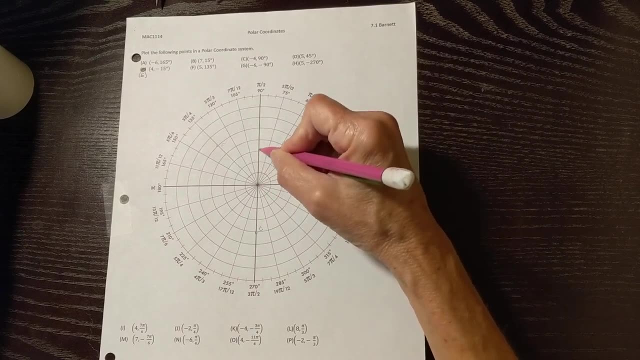 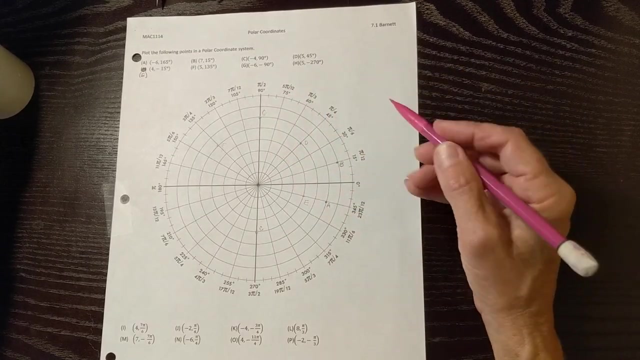 So we would move this direction. However, it is negative: 6.. So we're going to go the opposite way: 6 units, 1,, 2,, 3,, 4,, 5,, 6, and we will put G right there. H is 5, negative 270.. Where is negative? 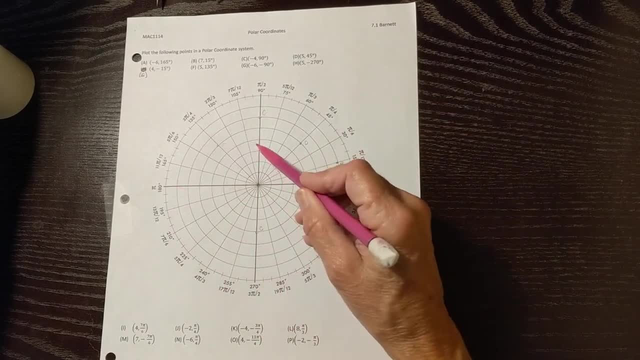 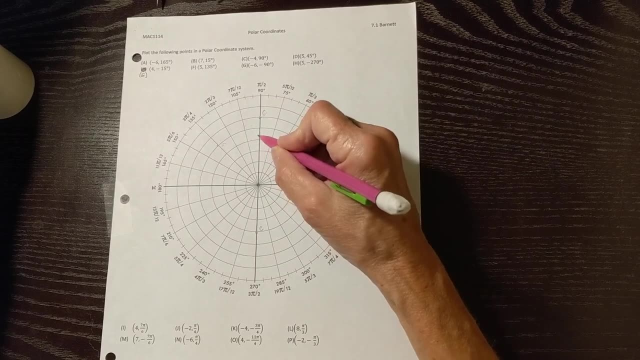 270?? Well, negative 270 is. this way It's the same thing as 90. So find negative 270. There it is- and go up 5.. 1,, 2,, 3,, 4,, 5, and this is where we will put H At the bottom of your sheet I've given. 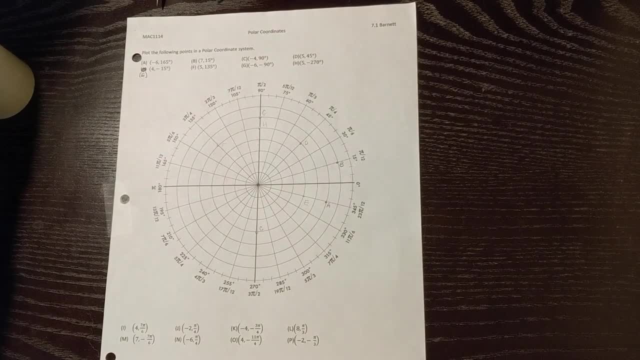 you more points to plot. However, they're not in degrees, They're in radians. So that's fine. We know how to do both of these things For 7 pi over 6,. first go to the angle 7 pi over 6, and it is. 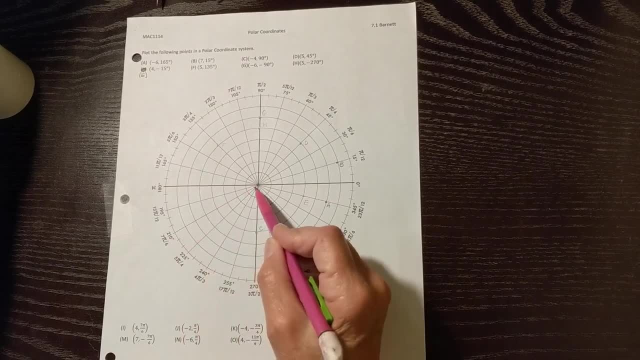 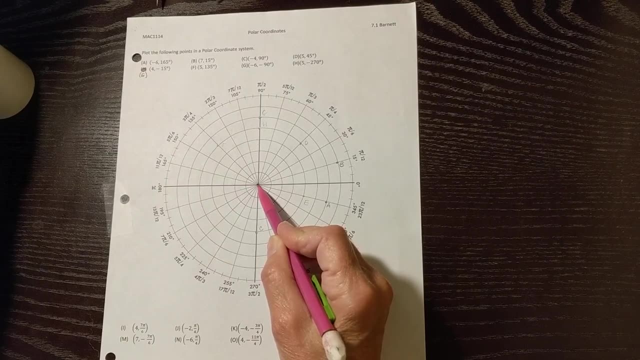 right here It's marked This is 7 pi over 6, and we're supposed to move 4 in this direction from the pole, the origin sort of. So we're going to go down 1,, 2,, 3,, 4 in that direction and put a point. 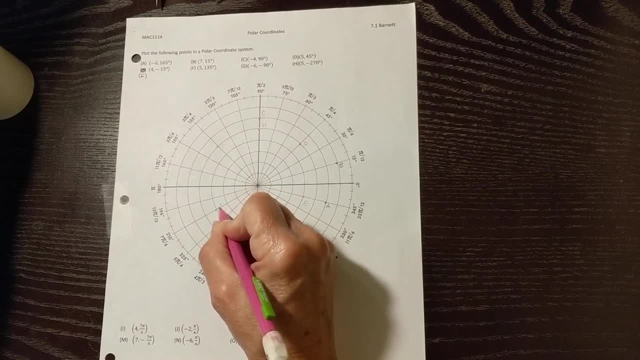 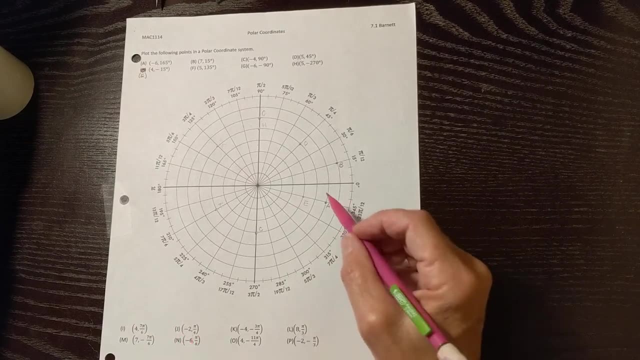 and that is going to be I. I okay, and then J is negative 2, pi over 4.. So go to pi over 4.. Right, here is pi over 4.. Since it's negative 2, we'll go in the other direction and that's. 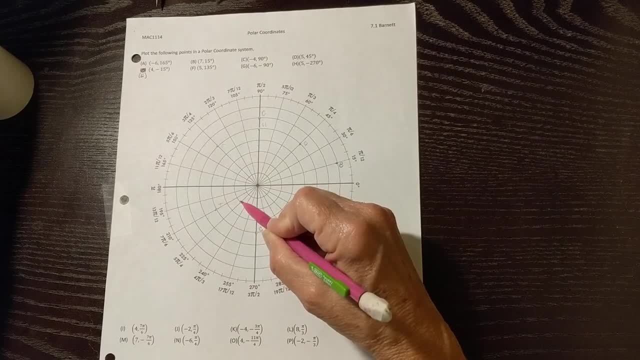 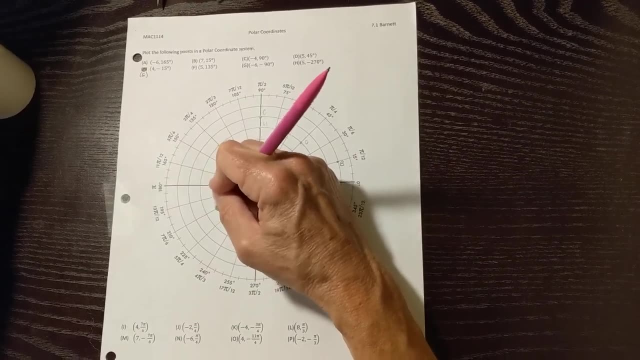 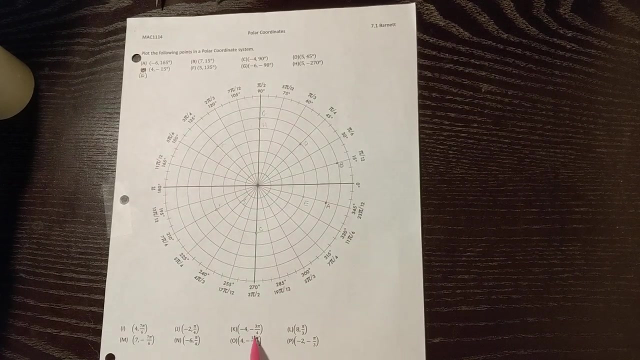 it opposite direction, so we're going to go down one, two in the opposite direction and that's where j is. last time i put little wings on my eye. it confused the class. they thought it was an h so i'm just going to label. i like that: um k is negative four. negative three, pi over four, so go. 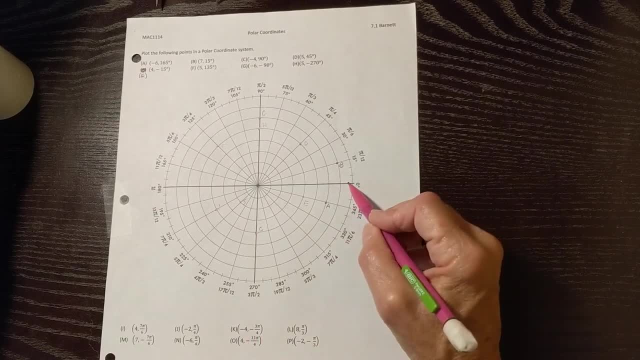 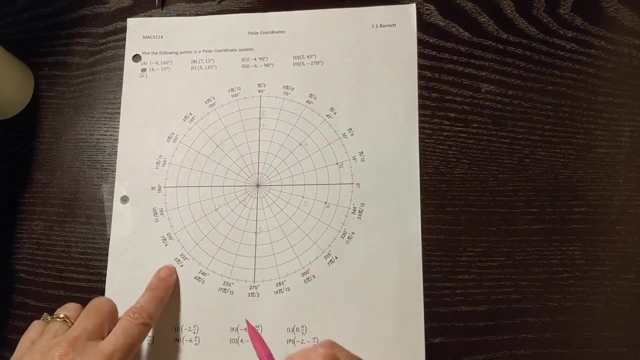 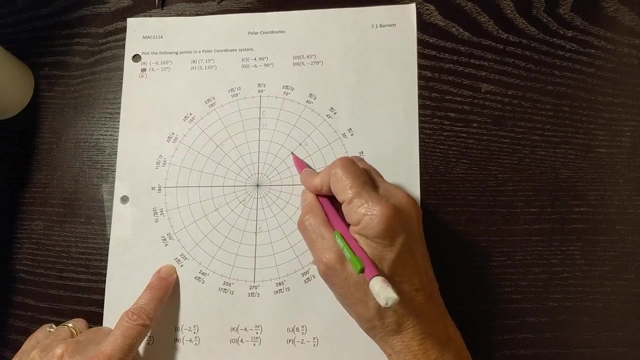 to the angle negative three pi over four. so this is negative pi over four. negative pi over two. negative three pi over four is right here. but it says to go negative four. so that means we'll go in the opposite direction. so we're going to go up one, two, three, four, and that is where k gets labeled. 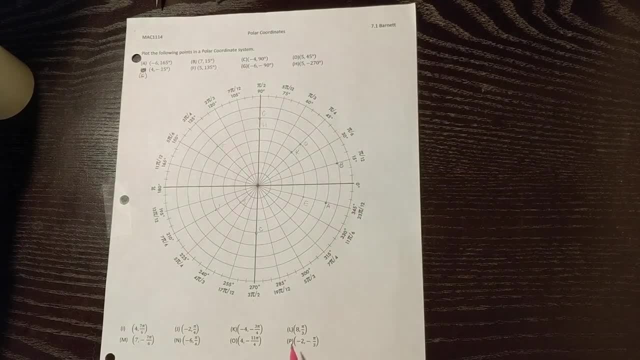 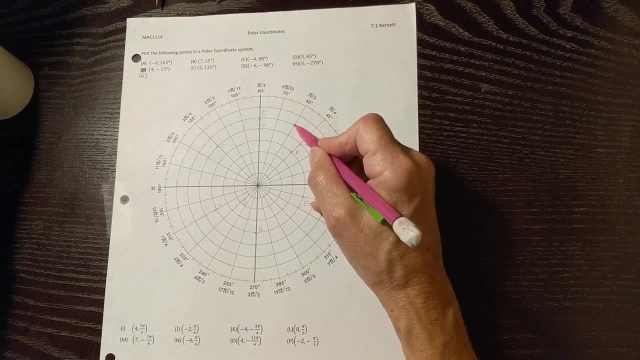 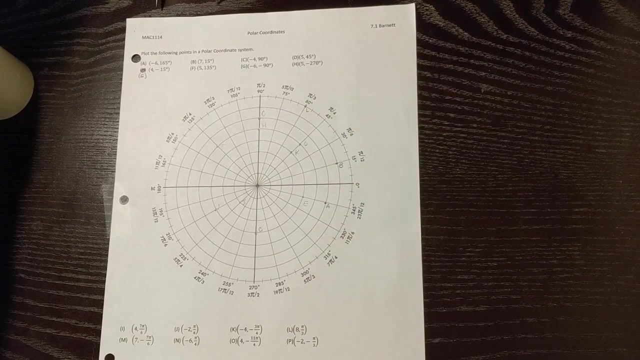 l is eight. pi over three. go to pi over three. here it is and we're going to go up eight. one, two, three, four, five, six, seven, eight. it's right here, and that is you point. l m is seven. negative pi over six. go find negative pi over seven. pi over six, okay. 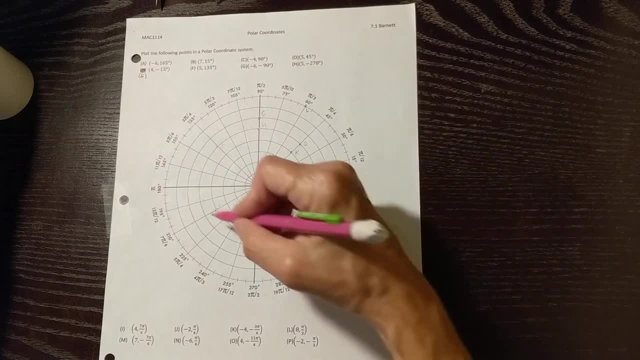 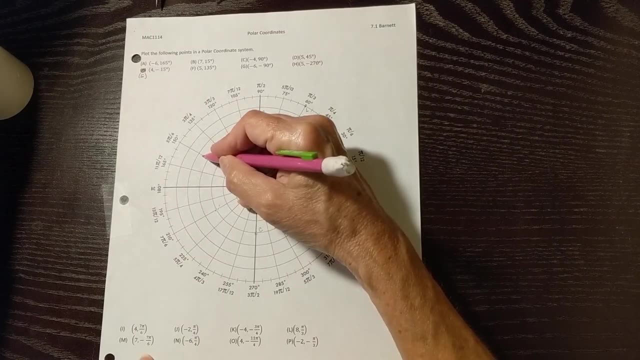 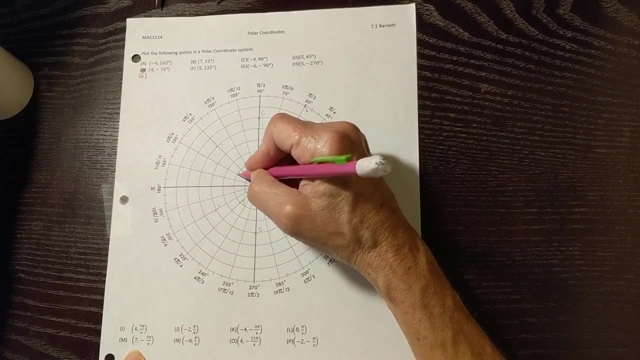 negative seven pi over six is all the way, all the way here at five positive five pi over six, that is negative seven pi over six. and then we're supposed to go seven units that direction. so go from the center of that direction: one, two, three, four, five, six, seven. 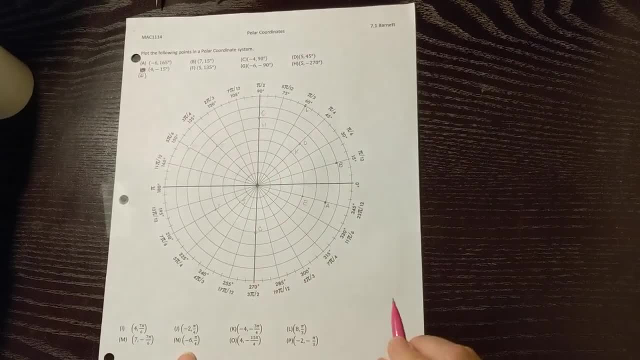 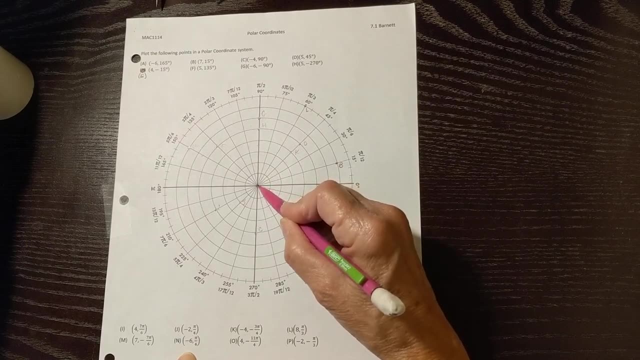 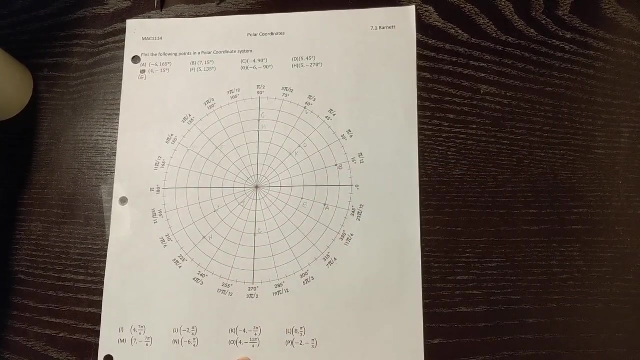 that is m? n is negative six pi over four. go find pi over four. here it is, go six in the opposite direction, because it was a negative number one: two, three, four, five, six, that's n? o is four, negative 11 pi over four. now this one you have to think about a little bit, because you don't. 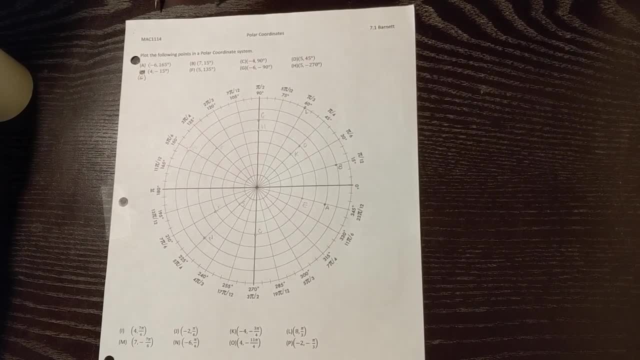 see negative 11 pi over four. so let's find something we can that's co-terminal. negative 11 over 4 plus 2 pi over 1 is coterminal, Just to make sure you can see it: negative 11 pi over 4. 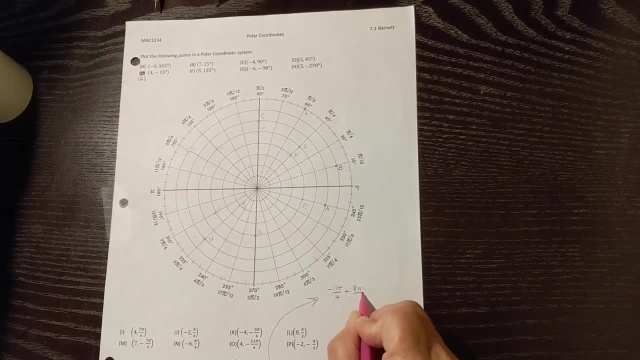 plus 8 pi over 4 is the same thing as plus 2 pi. Now they have a common denominator and I can add this is negative 3 pi over 4.. So negative 11 pi over 4 is coterminal with negative 3 pi over 4.. 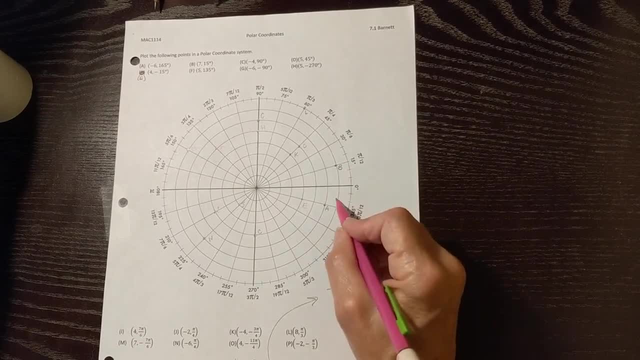 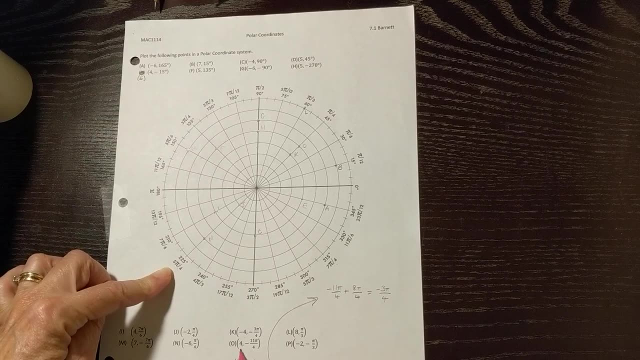 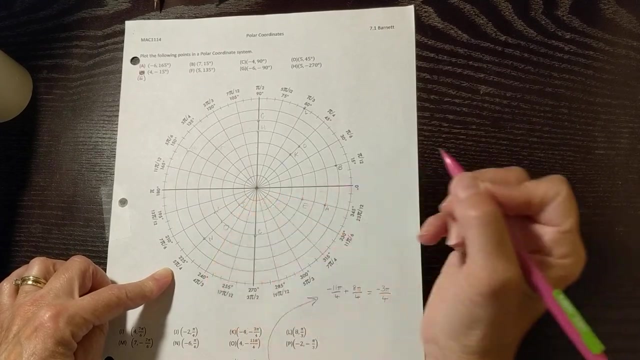 So go to negative 3 pi over 4.. So that is right here. right here is negative 3 pi over 4 at 5 pi over 4.. Go 4 units in that direction. So we're going to go 1,, 2,, 3,, 4, and that is where O will be. 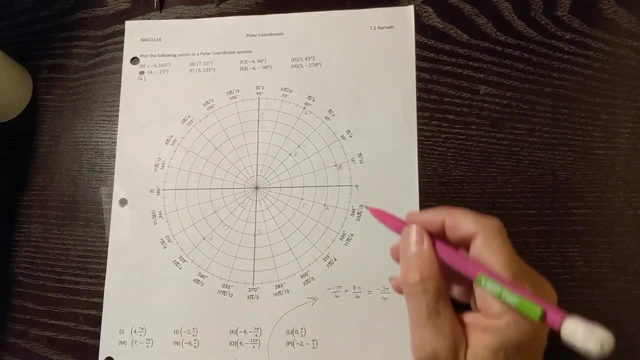 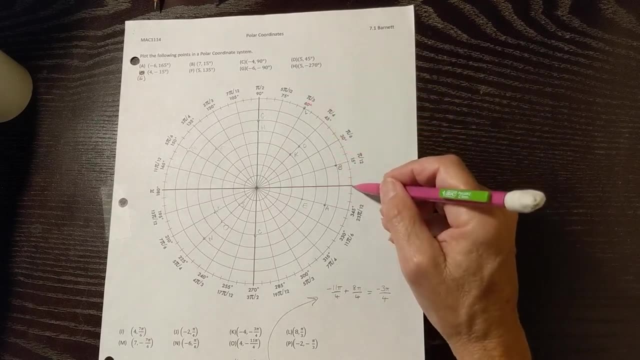 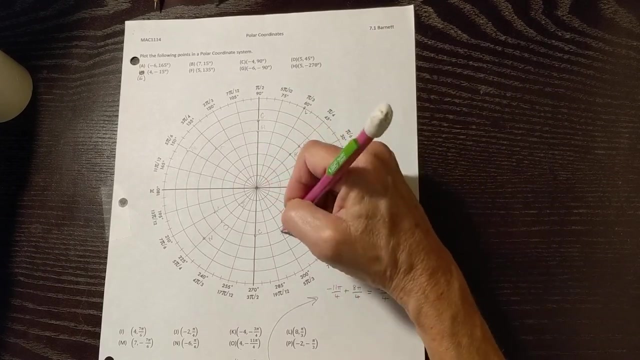 P is negative. 2, negative pi over 3.. Go find negative pi over 3.. So pi over 3 is this far up positive, so pi over 3. So pi over 3 is down here at 5, pi over 3. This is negative pi over 3.. And so this is the direction. 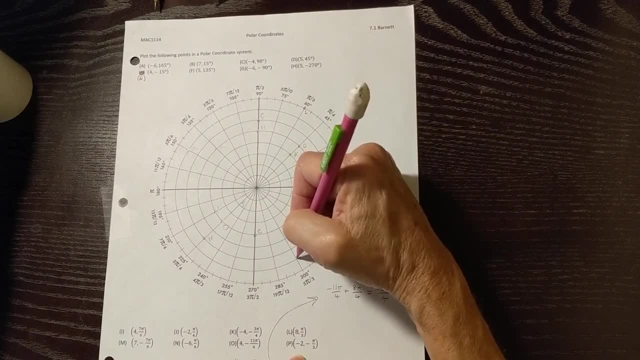 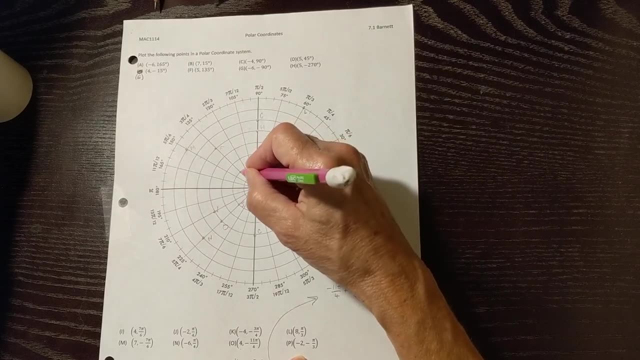 we would move However it says to move: negative 2.. So we're going to go the opposite direction from here. We're going to go up 1, 2, oops, sorry, I'm on the wrong one- 1, 2 at the 2, pi over 3.. 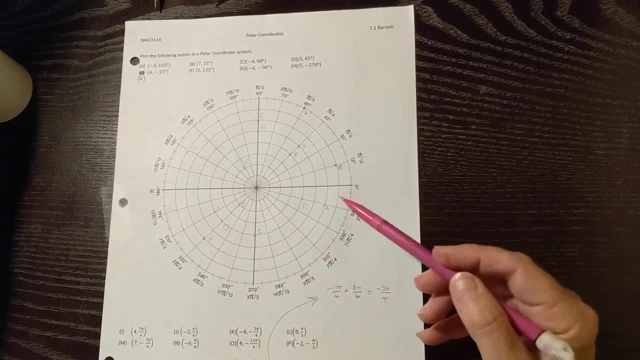 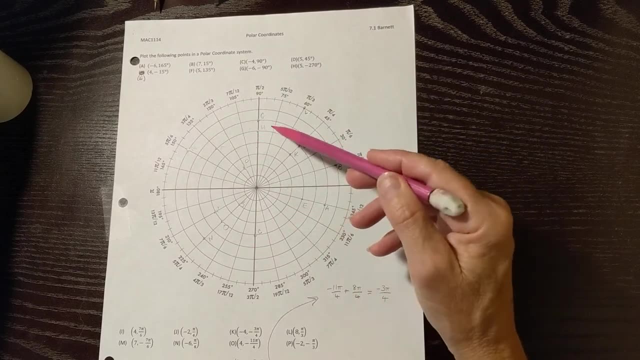 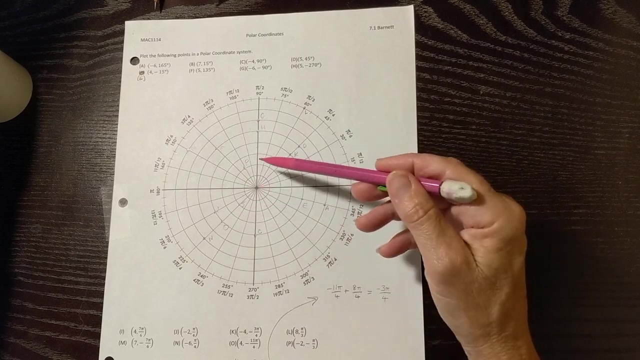 That is where point P is. So did I get all the points A, B, C, D, E, F, G, H, I, J, K, L, M, N, O, P? Okay, looks like we got them all. That is how you can. graph a point in the polar coordinate system.